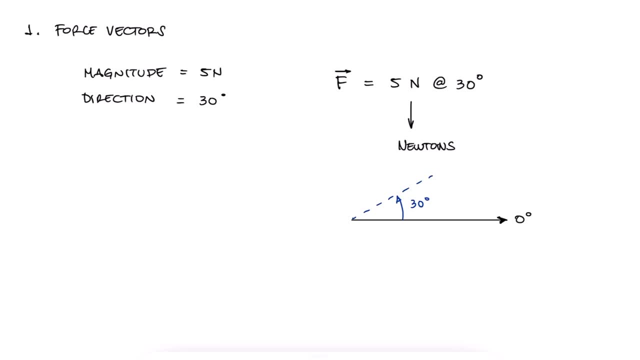 for statics, the angle or direction of a force vector can be with respect to any linear geometry of the setup. Besides this, notation vectors can also be used to calculate the direction of a force vector. A force vector can be represented with their three-dimensional components in Cartesian coordinates. 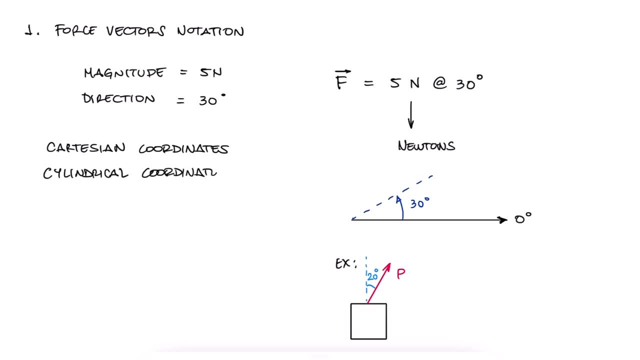 and- although we will cover this much later- in cylindrical or spherical coordinates too. A force vector can therefore be presented as its component's magnitude in the x, y and z axes, with the circumflex mark above the i, j and k directional unit vectors respectively. 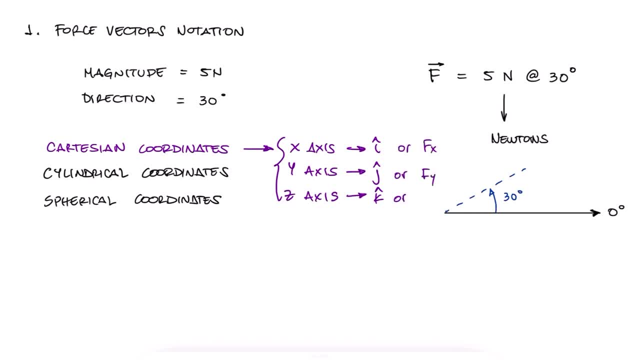 or separately, as f sub x, f sub y and f sub z. Finding these components is useful because what we will use to find the reaction forces, and with them the internal forces, is stating that a simple sum of forces in the x, y or z direction and later in the course. 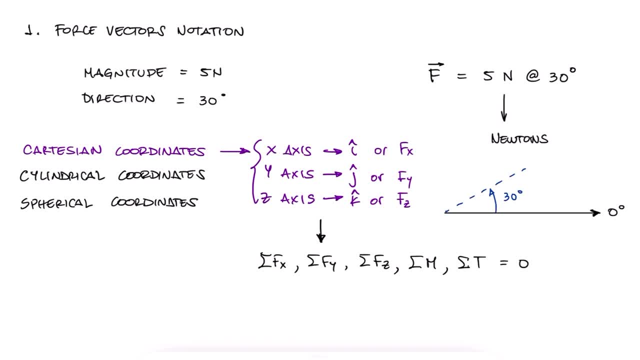 sum of moments and torques are equal to zero, since in most static scenarios the members of the structure are not accelerating. When given a force vector with its magnitude and direction, simple trig functions like sine, cosine and tangent are used to find the vector components. To find a force vector, 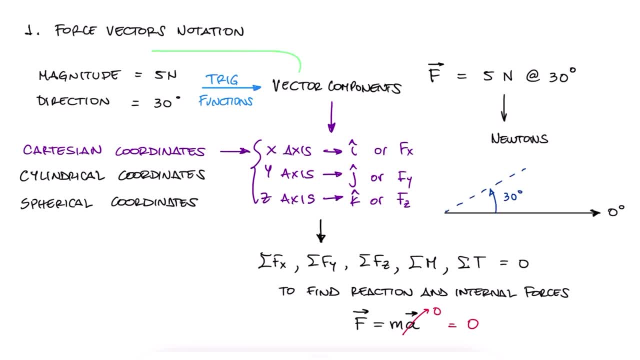 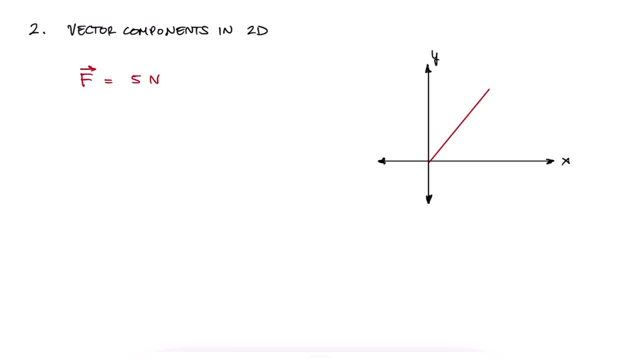 magnitude and direction based on its components, which is the opposite process. we use the Pythagorean theorem. If you want to review those basic concepts, you'll find some links in the description of this video. So let's start with a 2D force vector: F, 5, N in magnitude, at 53.13 degrees. This force vector 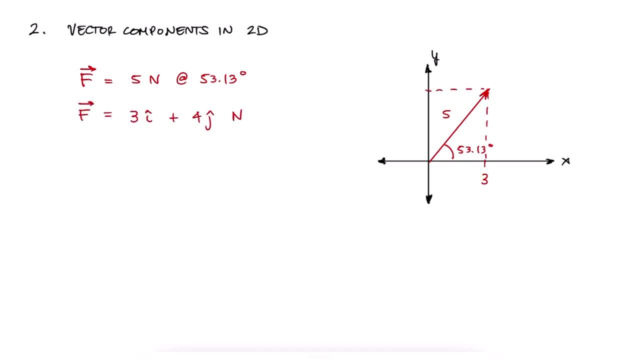 can be written as 3i plus 4j N, or we can say that Fx is 3 N and Fy is 4 N. To find these values here we are using the definition of sine, which is the length of the. 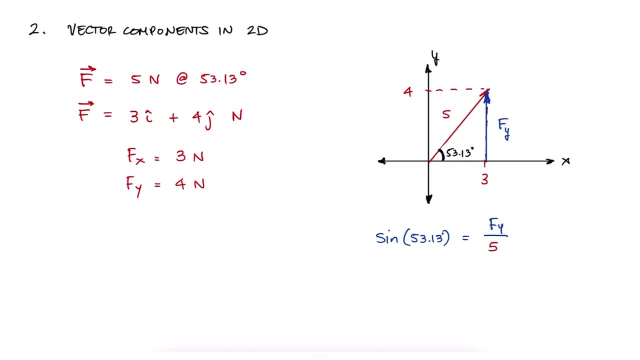 side opposite to the angle you know, over the hypotenuse, and cosine, which is the length of the adjacent side to the angle you know, over the hypotenuse. If, in this case, sine of 53.13 is Fy over the magnitude of F and cosine of 53.13 is Fx over the magnitude of F, then Fy is F sine. 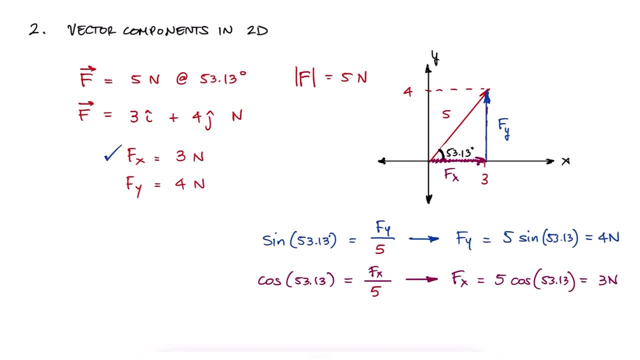 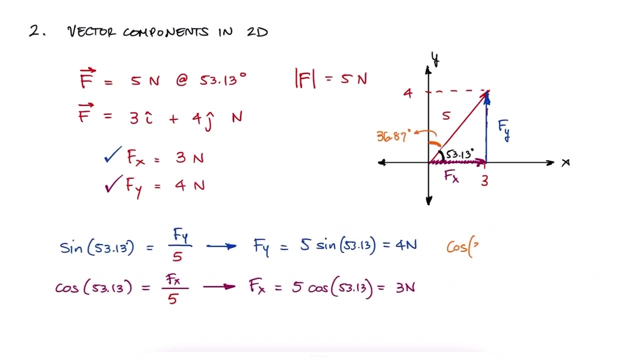 of 53.13.. Now I say in this case because sine is not necessarily the Y component and cosine the X component. If we had been given the complementary angle 36.87, then Fy would be F cosine of 36.87 and Fx would be F sine of 36.87.. Notice that in the first case I used sin. 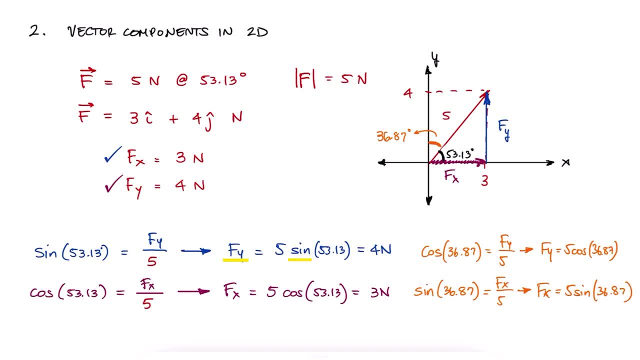 for Y and in the second sin for Y, but later with a queen, since sine isит hasn't been a sine, so it's not a sine component. Next up, ücks, we are looking at the housed Aristotelian geometry, which deems to beей tout complex If we 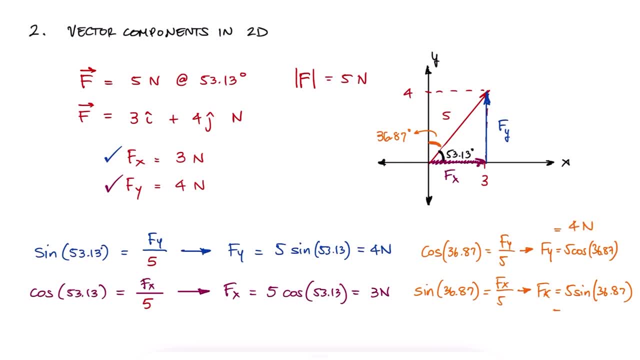 are looking at the housed Aristotelian geometry, we are afraid we are closer to the theorem round trouve How to for x. but this of course matches our values, since the sine of theta is equal to the cosine of the complementary angle. 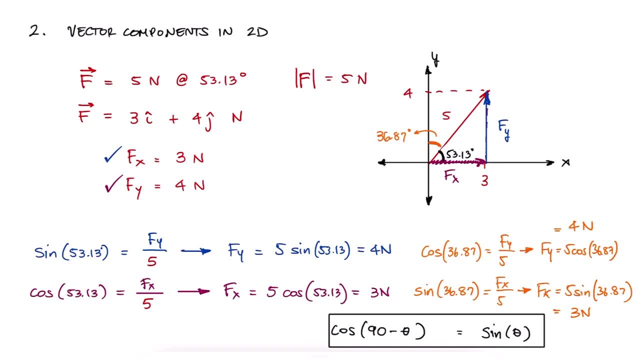 This means that, depending on the angle you are given or the angle you can measure, sine and cosine can be used to find any of the components. This is obviously especially true for 3D vectors, as there will even be z components, so of 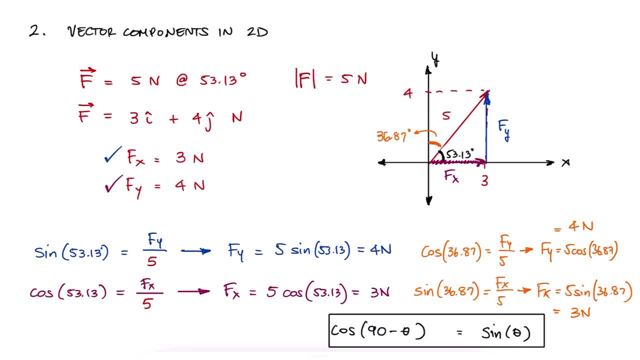 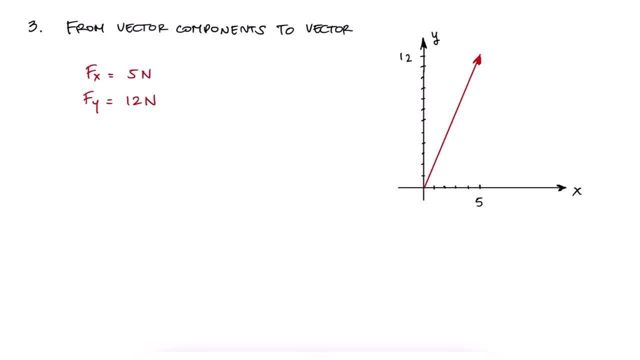 course we cannot generalize y and x for sine or cosine. From the components of a vector. we can also find the vector's magnitude and direction, Since the components are orthogonal, meaning that they form a 90 degree angle between them. we can use Pythagoras to find the hypotenuse, which would be the magnitude of the vector. 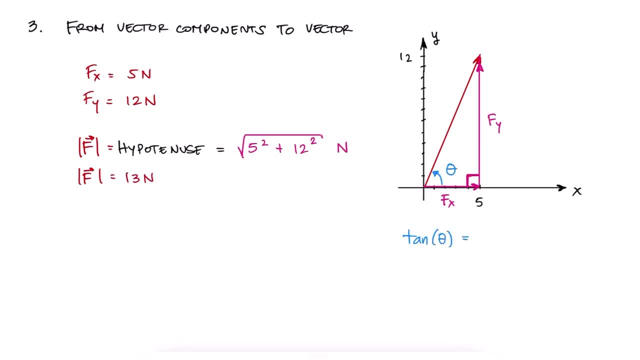 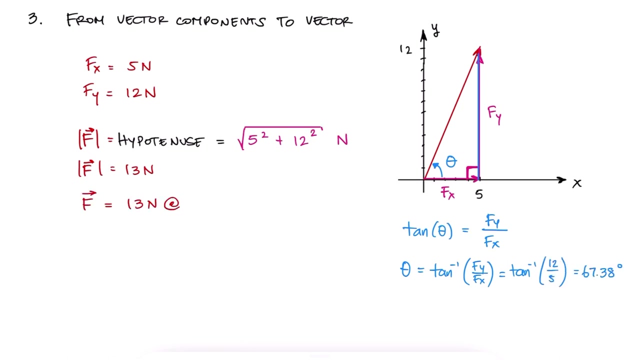 To find the direction of the vector, we would use the trig function tangent, which is equal to the length of the opposite side of the given angle over the length of the side adjacent to that angle, and therefore fy over fx. The angle would therefore be the arctangent of fy over fx. 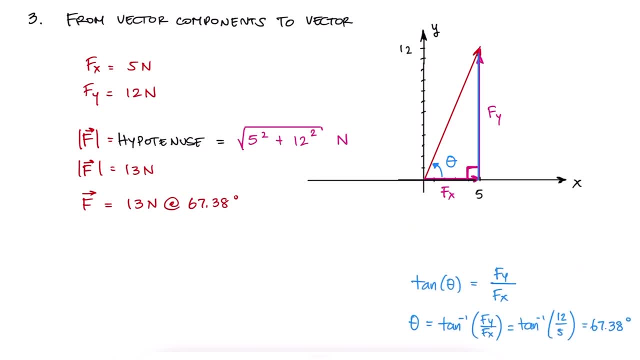 Now, this angle can be tricky, since if we had, for example, fx equal to minus 5 and fy equal to minus 12, solving for the angle mathematically would still give us a value between 0 and 90 degrees, when in fact we know that the angle from the positive direction 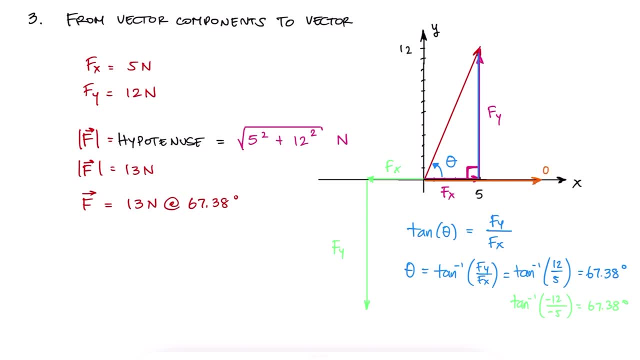 of the horizontal line which I just mentioned was the absolute reference for angles would be between 180 and 270 degrees. You can check out a trig-related video link in the description below if you want to brush up on this. but for static scores purposes, just remember that you need to identify the 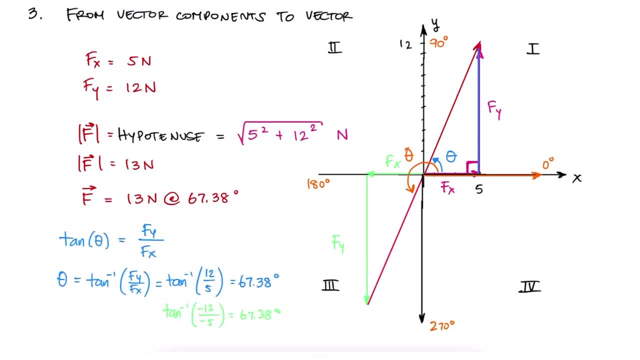 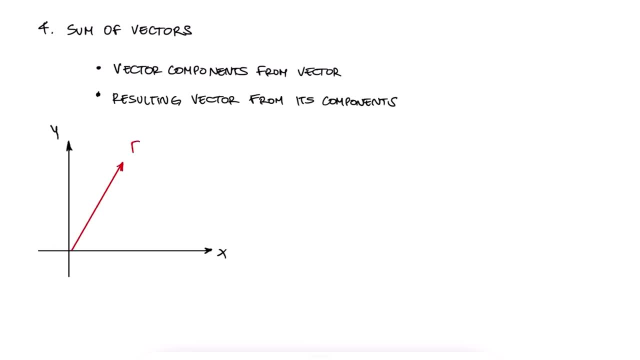 quadrant in which the resulting vector is pointing towards. We use these two concepts, decomposing vectors and finding the resulting vector from its components- when adding vector forces. Notice that the sine of 30, which is the angle we were given, is opposite over hypotenuse. 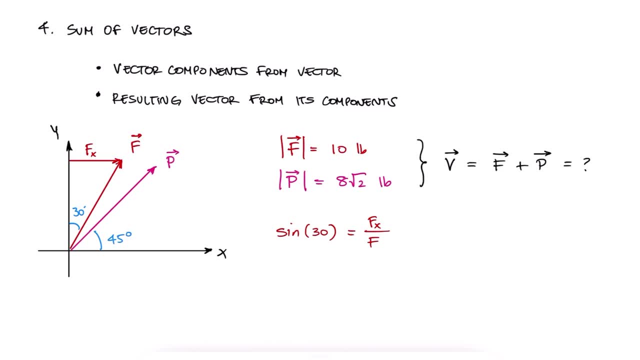 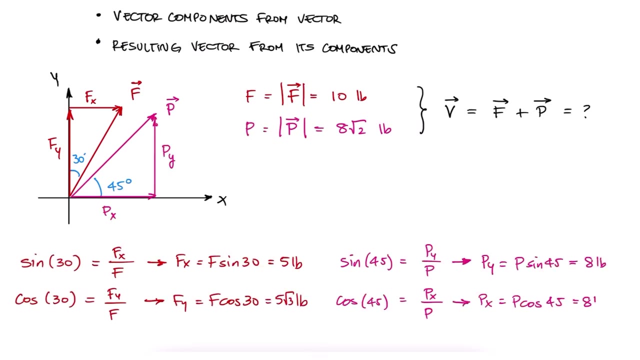 in this case fx over fx, And cosine of 30 is adjacent over hypotenuse. in this case fy over f. So fx is using sine instead of cosine, as opposed to the example. before Doing the same for p, and now, with the components of f and the components of p, we can add forces. 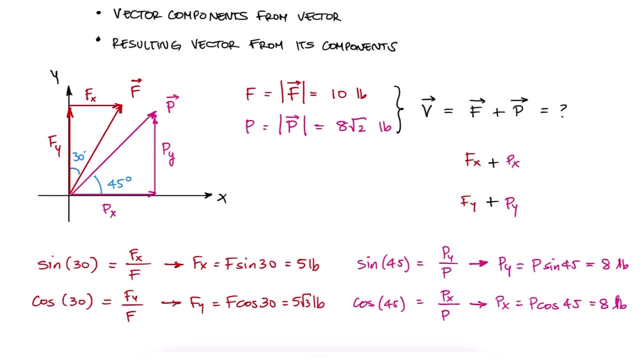 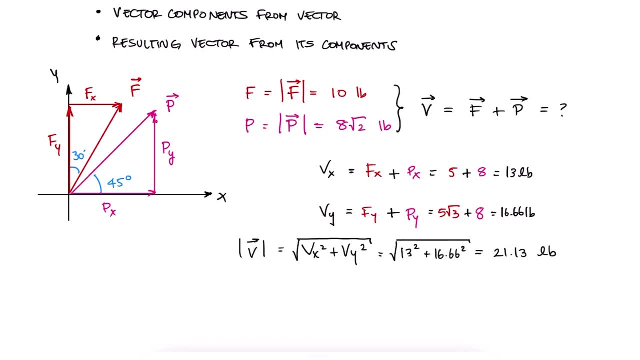 in the x direction and forces in the y direction, to have the components of the resulting force v. To find the magnitude of v we use the Pythagorean theorem and with the tangent we find that the resulting vector is angled at 52 degrees. 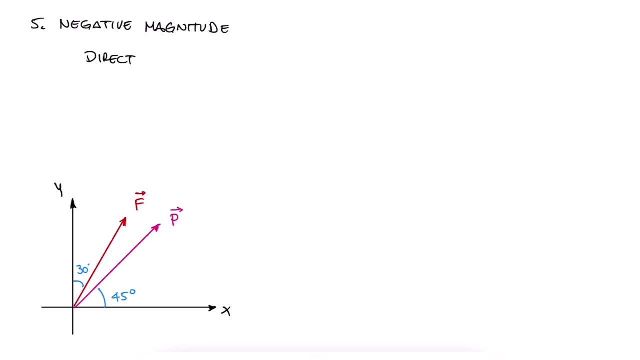 Worth pointing here is that the direction and the orientation of a vector are two distinct properties. Adding these two vectors graphically so that we can identify our resulting vector v, we can see that a vector of minus 21.13 pounds at 232 degrees is equivalent to the force. 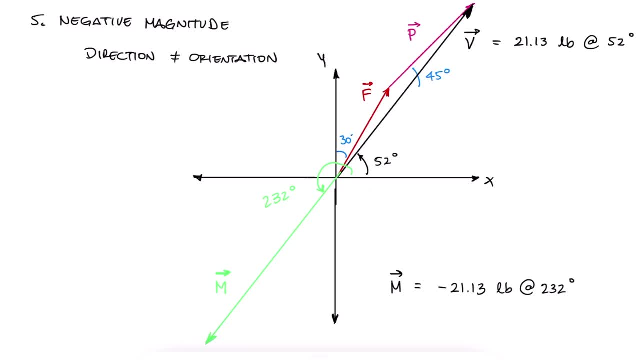 vector v we just found. This will be very important when finding reaction and interaction. This will be very important when finding reaction and interaction. If the direction of a vector you're trying to find is not obvious from the setup you're given, you can always assume a direction and if the magnitude results in a negative, 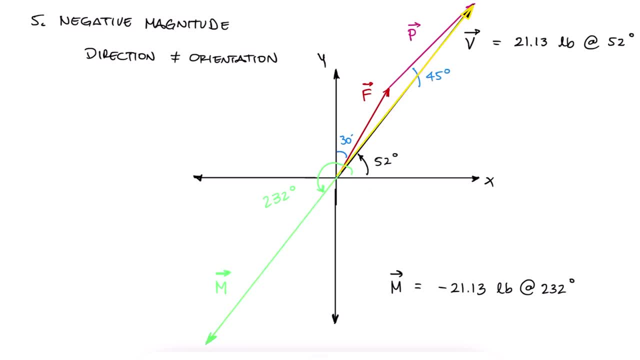 value. it means that the direction was the opposite of what was assumed. We'll talk more about which directions to always assume to avoid extra work or confusion in later videos. These same trig functions and Pythagorean theorem are used when dealing with 3D vectors. The components of a given vector can be found using the Pythagorean theorem. The components of a given vector can be found using the Pythagorean theorem. The components of a given vector can be found using the Pythagorean theorem. In this case, we can use the Pythagorean theorem to find the direction of a vector and the. 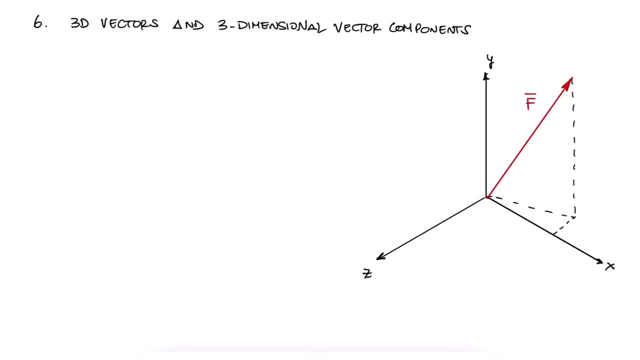 direction of a vector can be found using sines and cosines, in this case with two angles and, of course, just one magnitude value. The y component of f would be equal to 50 cosine of 30,, since the y component is the 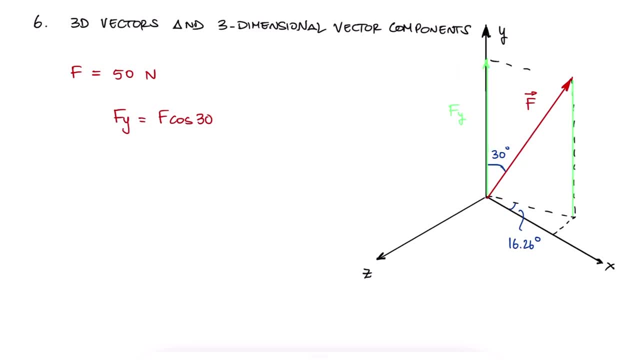 adjacent side, and therefore cosine, of the 30 degree angle. On the other hand, the opposite side of the 30 degrees, which is at the top but also at the bottom, that is, 50 sine of 30, would be the hypotenuse of the right triangle. that 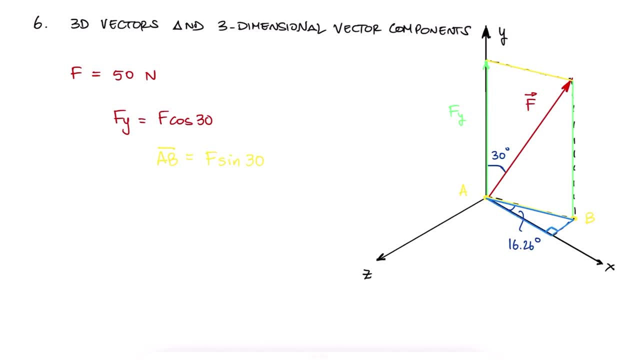 is found on the horizontal plane. With that hypotenuse and the angles shown, we can decompose that into the x component of f with 25 cosine of 1626 and into the z component of f with 25 sine of 1626.. 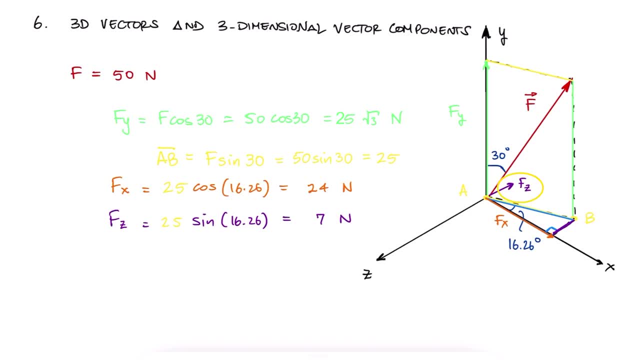 When finding these values, you have to remember that the component of z is going in the negative direction of the z-axis. So if we're presenting the vector f with the i, j and k notations, we're going to find that the y component of z is going in the negative direction of the z-axis. 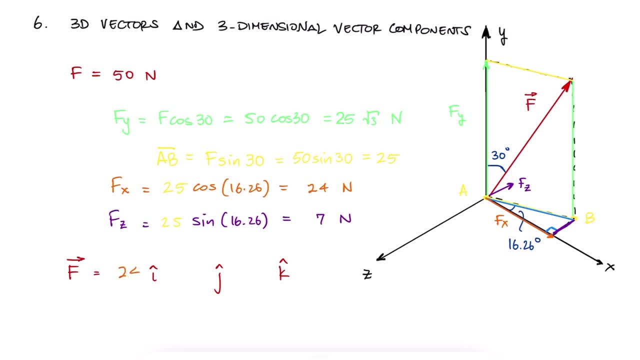 So if we're presenting the vector f with the i, j and k notations, we're going to write it as 24i plus 25, square root of 3j minus 7k. Now, if we're only writing its components fx, fy and fz, fz can be either negative. 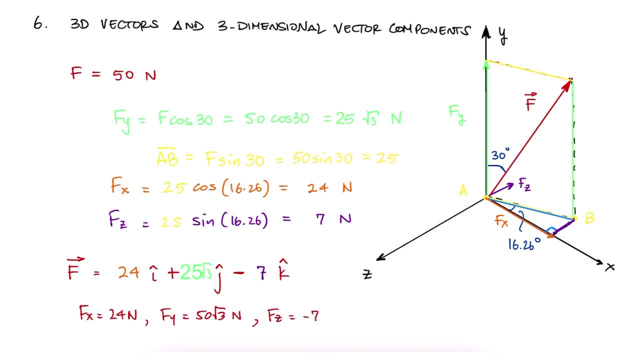 if there is no graphical representation of where the vectors are located, so that anyone reading the information knows that the z component is negative or positive. if the vector component fz is shown like it is in this case here, Remember that a vector in one direction with a negative sign is the same as a vector with 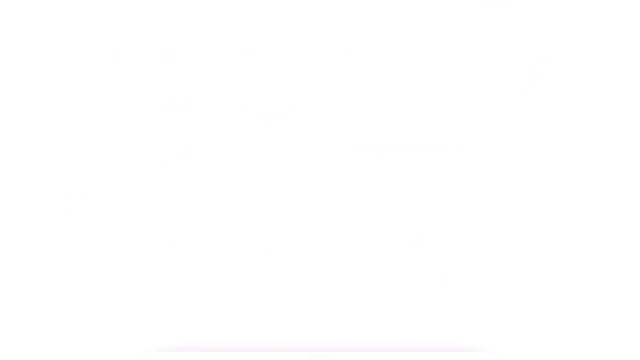 a positive sign in the opposite direction. So now let's take a look at a brief example where we put into use what we've covered here today, For the force vectors F and P shown what is the magnitude and direction of an additional force V, so that all three forces added together would be equal to zero. 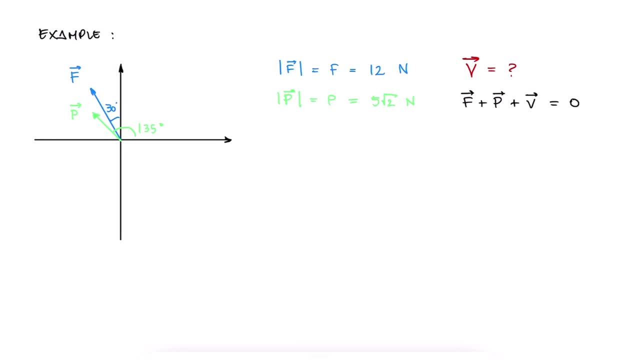 Before watching the solution to this example, pause this video and try working on it and solving it yourself. We know that when adding vectors, we add their components separately, and if we want the resulting vector to be zero, it means that its components are also zero. 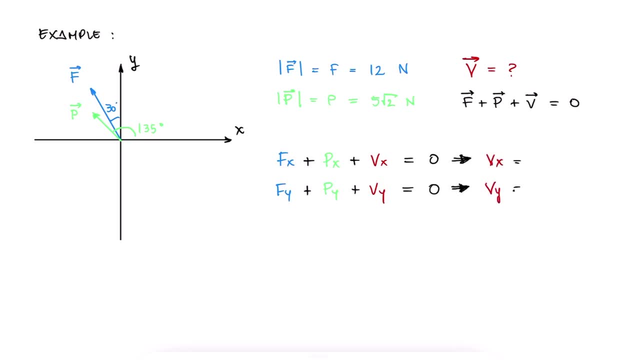 To find the magnitude of V, we will first need to find its components Vx and Vy, And to do that we need to find the components of forces F and P. The x component of F will use the trig function sine, since that component is the side opposite. 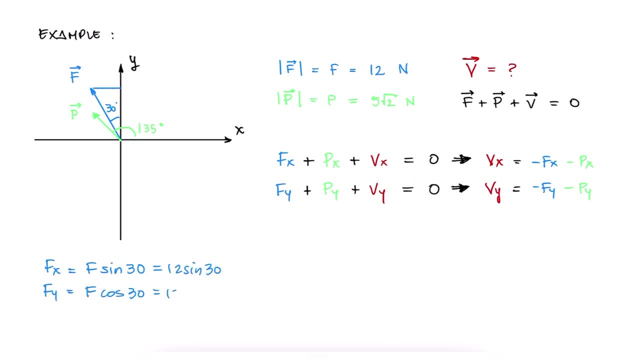 to the angle 30.. And Fy is equal to F cosine of 30.. And since the x component of F is pointing left, we know that Fx is negative For vector P, we will use a right triangle that has an angle equal to 180 minus 135.. 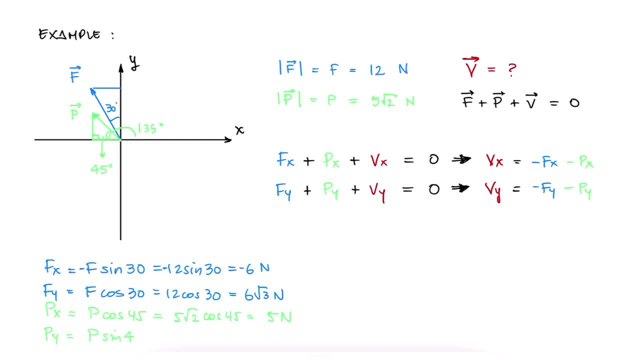 Px would be the adjacent side and Py the side opposite to that angle. And again, since the x component is pointing in the negative x-axis direction, Px will be negative. Substituting these values, we find the components of vector V. 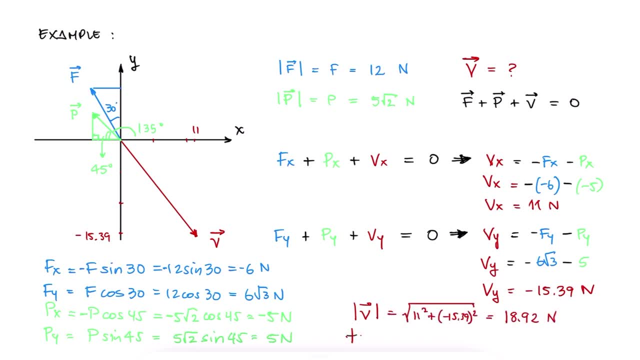 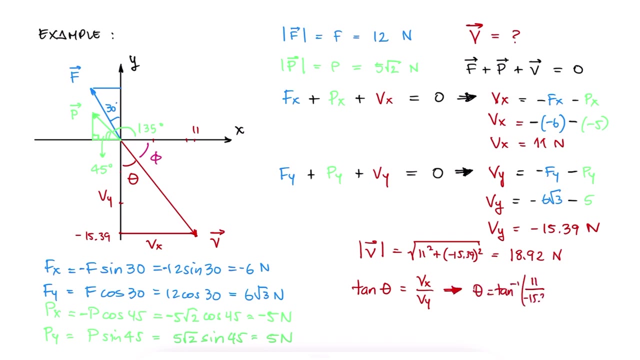 With Pythagoras we find its magnitude and with tangent the angle of orientation. The angle that we define as theta can be that between the vertical line and the vector, or between the horizontal line and the vector. In the first case, we would have the x component over the y component, and if we're just looking, 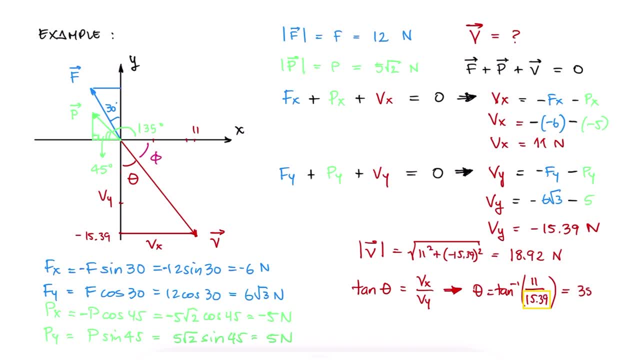 at the lengths of a triangle, they would both be positive, including Vy, And in the second case we would have the x component over the y component. and if we're just looking at the lengths of a triangle, they would both be positive, including Vy. 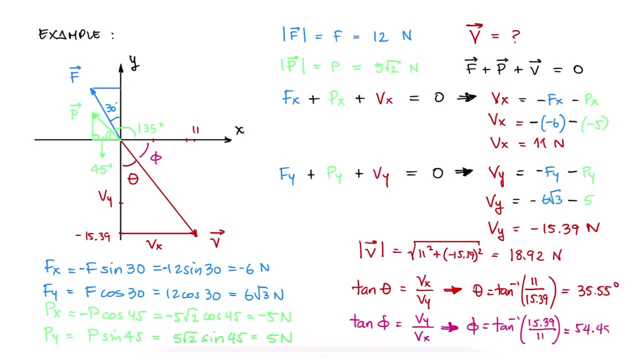 Tangent of phi would be equal to Vy over Vx. The overall direction, meaning the value of the angle with respect to the horizontal line, would therefore be 270 plus theta or minus phi. The process we've done here today is very similar to what we will do to find reaction. 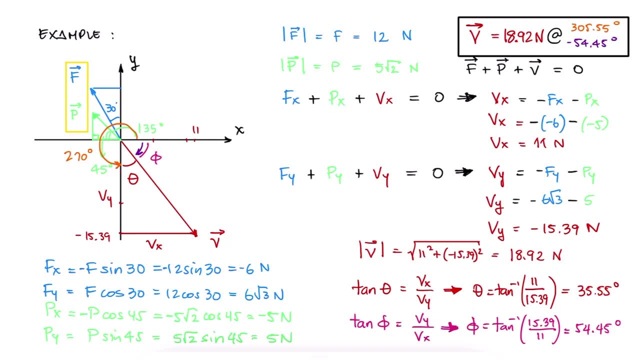 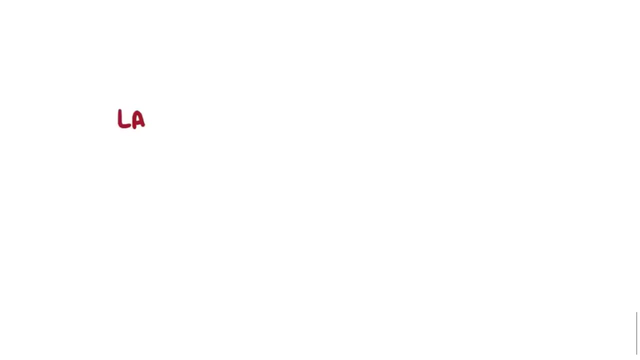 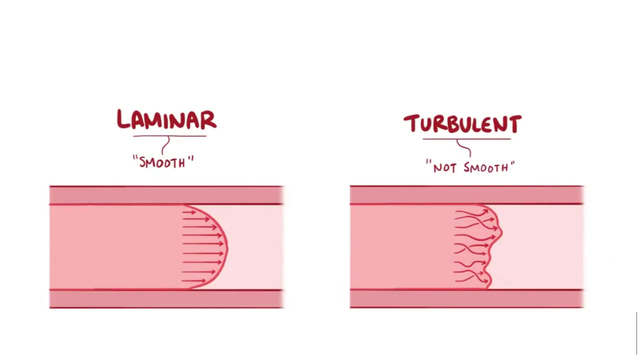 Laminar means smooth, and so laminar blood flow is blood that's flowing smoothly through the vessels. Turbulent flow, on the other hand, is when the blood is not flowing smoothly, and we can figure out if blood is likely to be laminar or turbulent by finding its Reynolds. 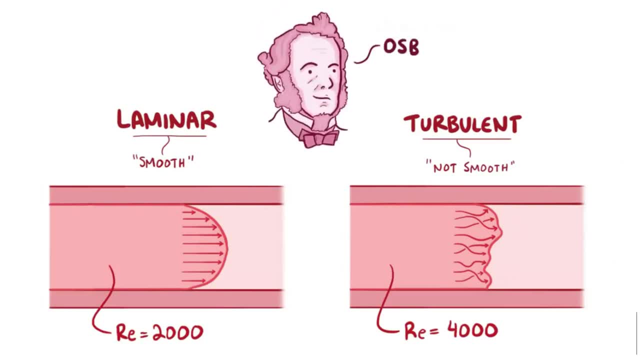 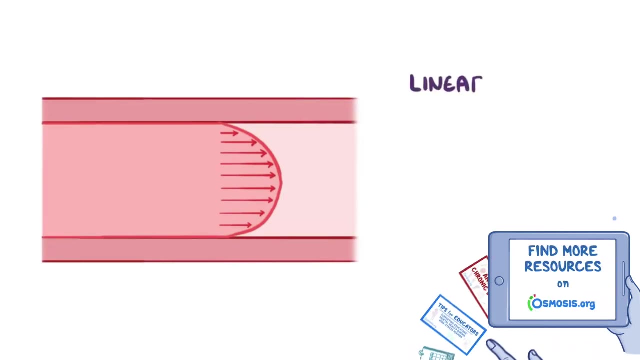 number, or RE, which is named after Osborne Reynolds, a Victorian scientist who not only studied fluid dynamics, but is a man who knows how to rock a beard and bowtie. Now, if everything's moving like it should and blood flow is laminar, then the linear